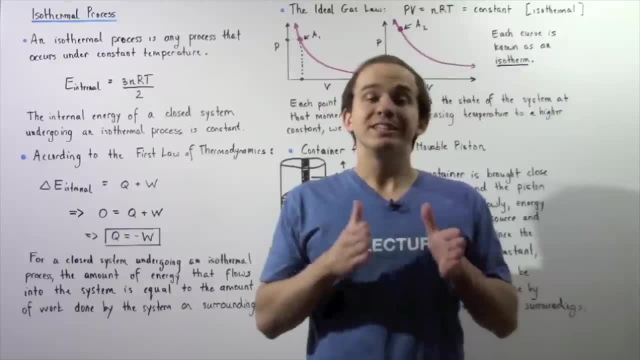 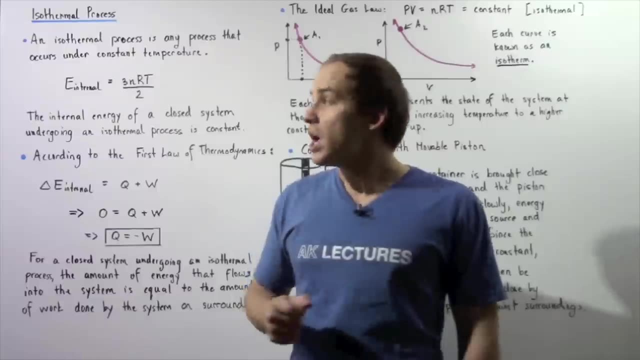 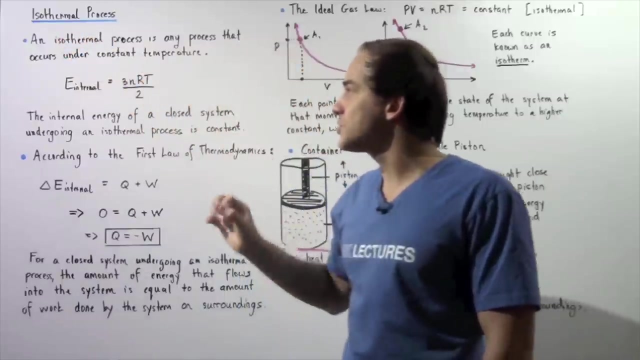 into our system as a result of a change or a difference in temperature, and W is the work done on or by our gaseous system. So, because we're assuming our closed gaseous system is undergoing isothermal process, that means that this remains constant. And if this remains constant, then the 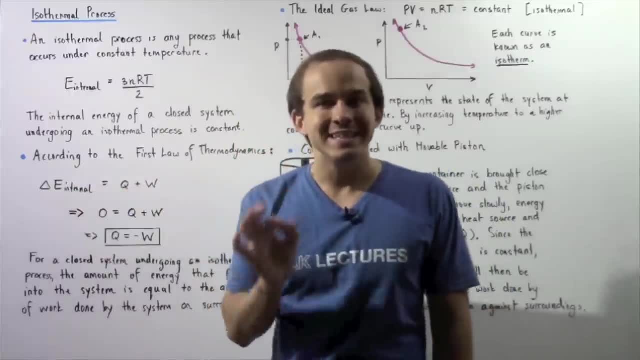 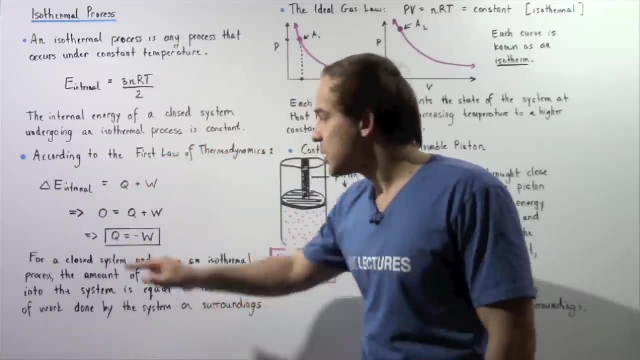 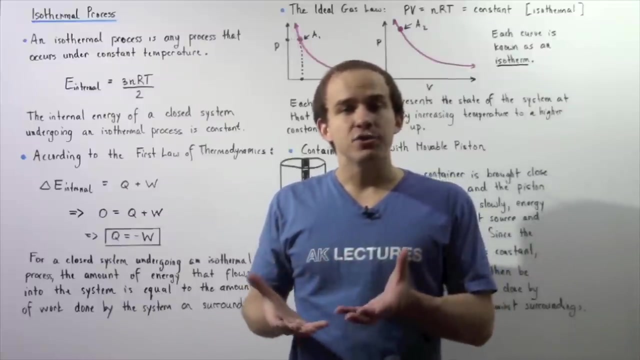 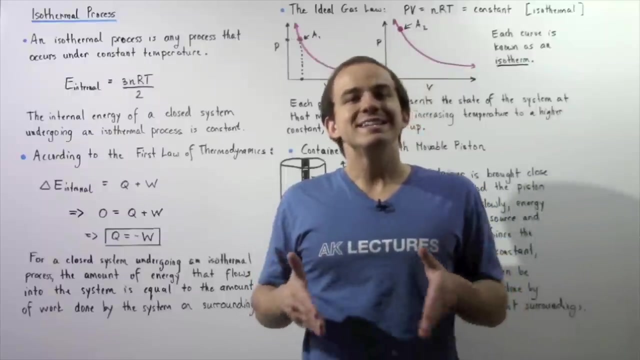 change in internal energy remains zero. So zero is equal to the sum of Q and W. That implies that Q is equal to negative W. That means that the amount of energy that flows into our closed gaseous system as a result of a difference in temperature is equal to the work done by our gaseous system. 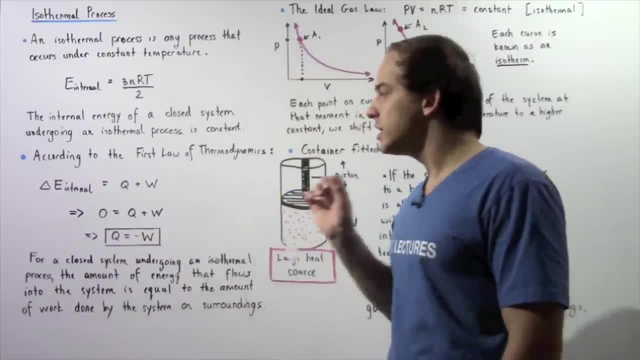 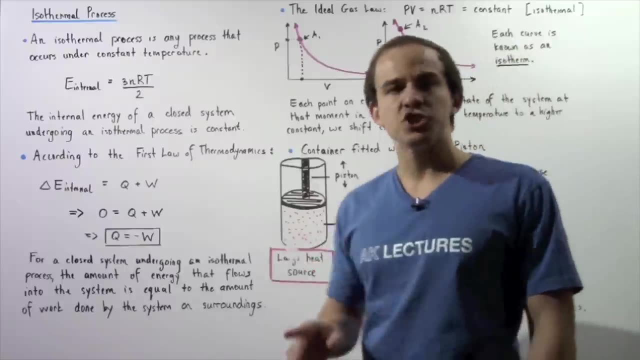 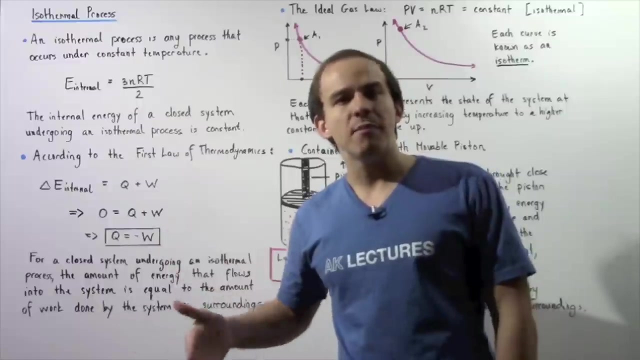 on or by our gaseous system. So that means that the change in internal energy remains zero. So once again we conclude that for a closed ideal gas system undergoing an isothermal process in which the temperature remains constant, the amount of energy that flows into the system as a result of 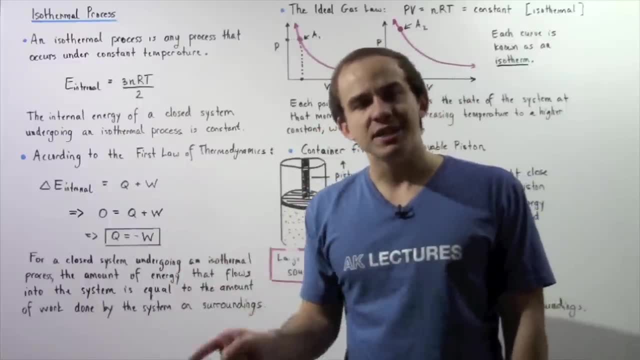 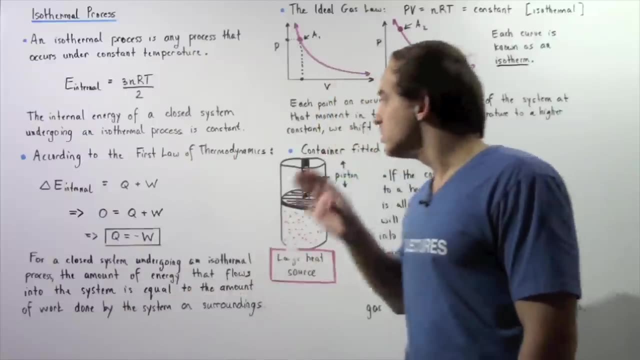 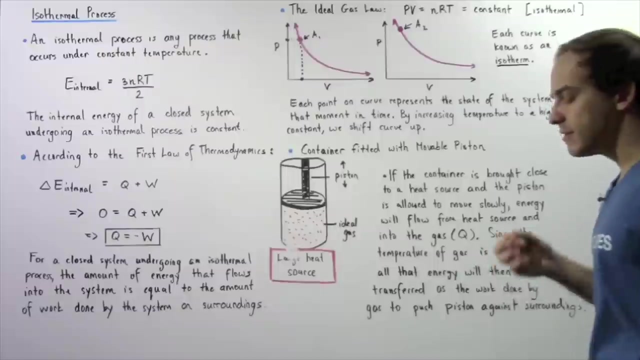 a difference in temperature between the system and the surroundings is equal to the work done by the system on the surroundings. So let's recall that the change in internal energy remains zero. So let's recall the ideal gas law. The ideal gas law states that the pressure times the volume. 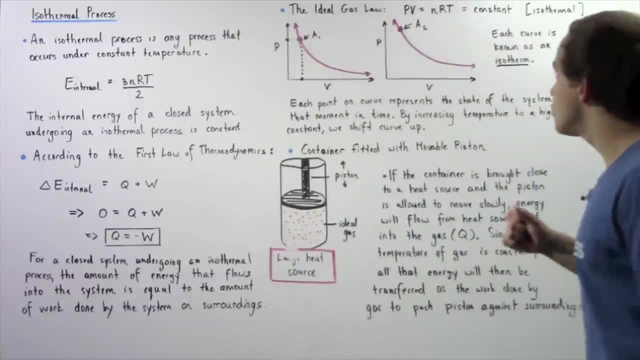 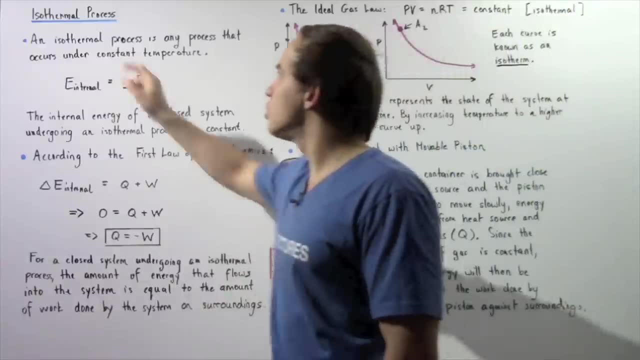 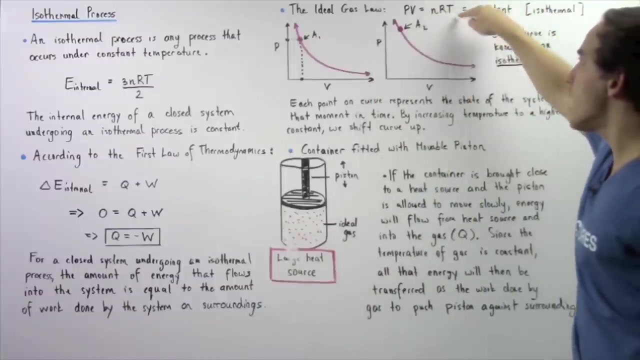 of our closed gaseous system is equal to the product of N, R and T. Now if we're dealing with a closed system that is undergoing an isothermal process, the N is constant and the T is constant. So that means the product of P times W also remains constant as long as the temperature. 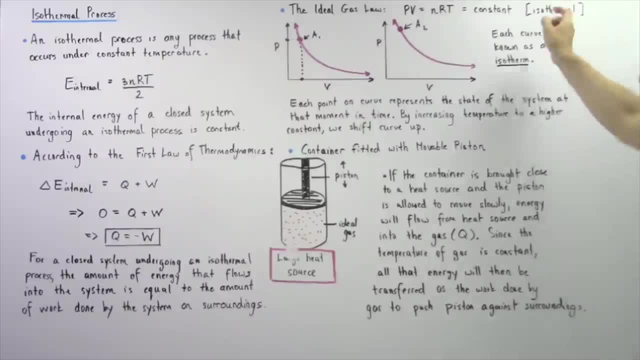 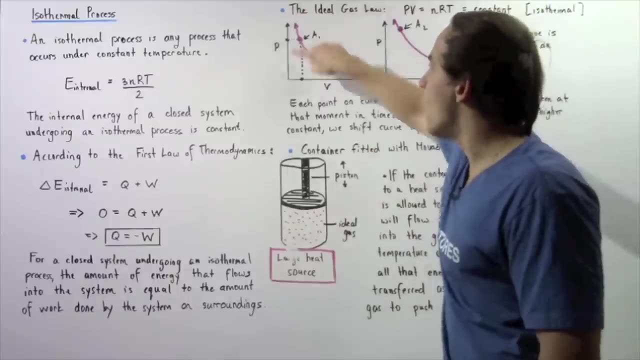 we're dealing with an isothermal process, So let's plot this on the x-y plane. So if we plot this on the x-y plane, the y-axis is the pressure and the x-axis is the volume And we obtain the. 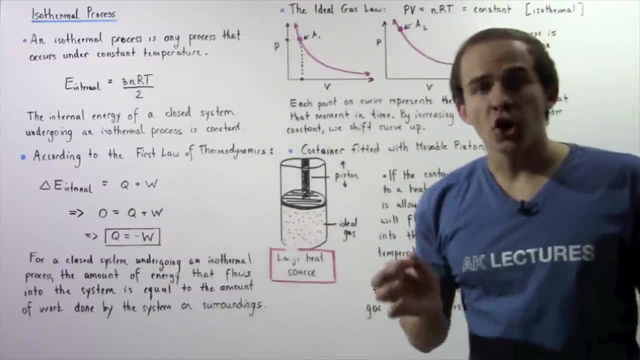 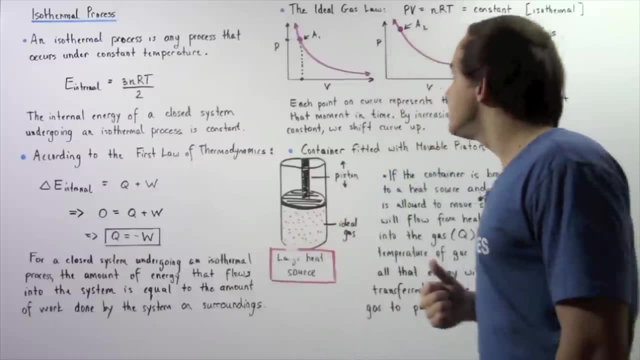 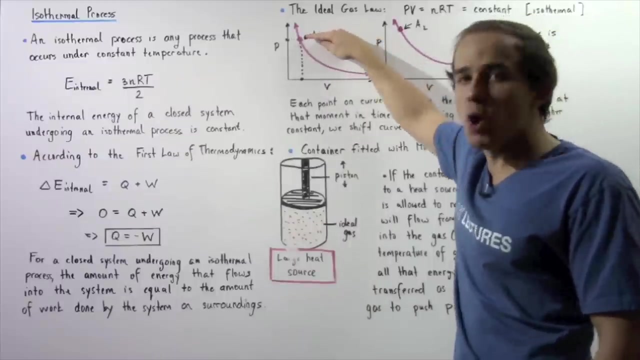 following curve. Now each point on the curve represents the state of the system at that particular moment in time. For example, if we examine this curve and we choose a point- let's call it point A1,, then at this moment in time the pressure is given by this quantity. 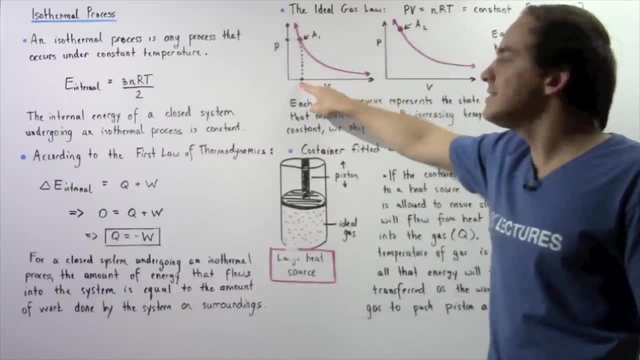 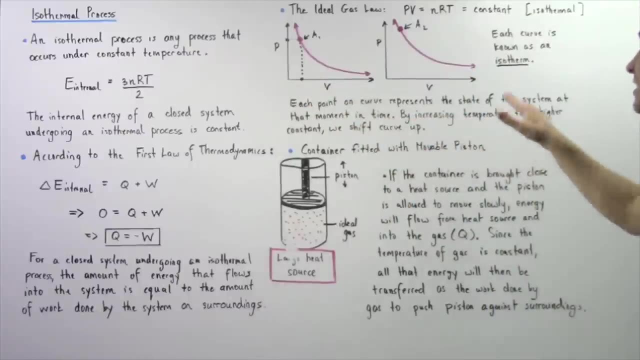 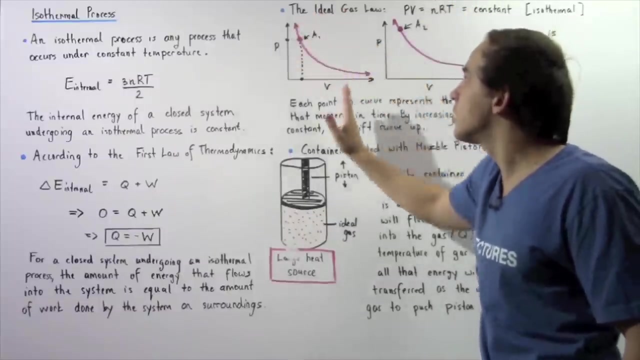 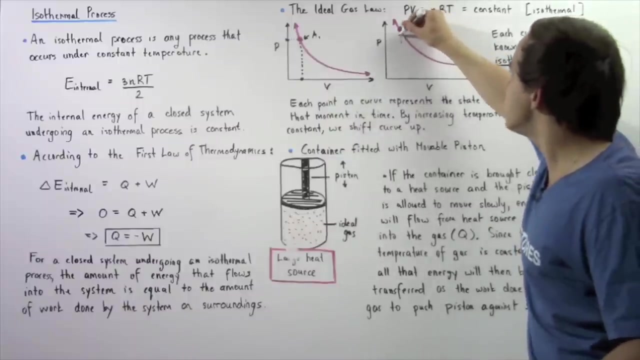 and the volume of our gaseous system is given by this quantity. Now notice: by increasing the temperature to a higher constant, we increase this entire constant. So that means we shift this entire curve upward, as shown. And so now at our point A2, the new volume is given by this: 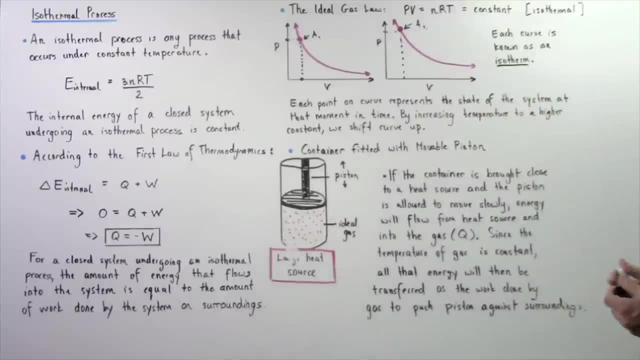 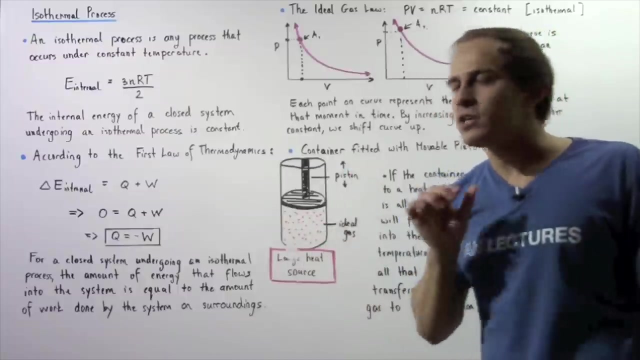 quantity and the new pressure is given by this quantity And each one of these curves is known as an isotherm. So notice the isotherm. the curve will drop down, will shift downward if we decrease the pressure. If we decrease the pressure, this constant decreases. 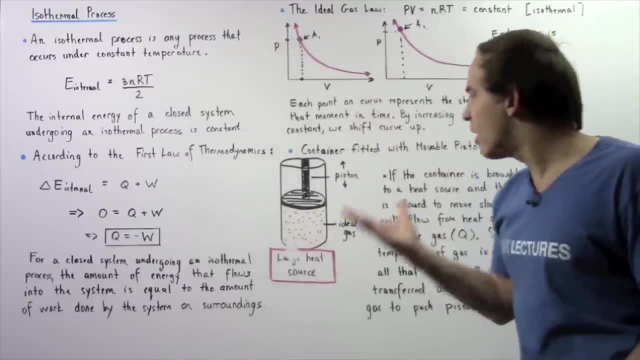 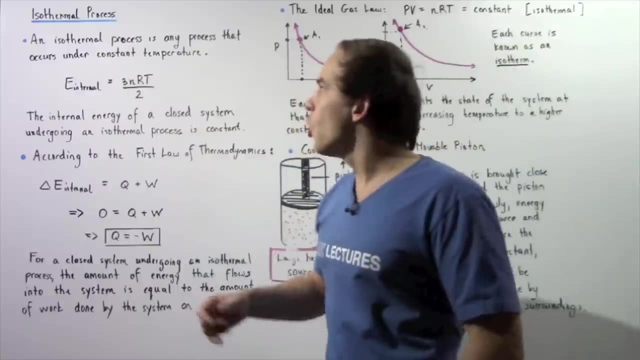 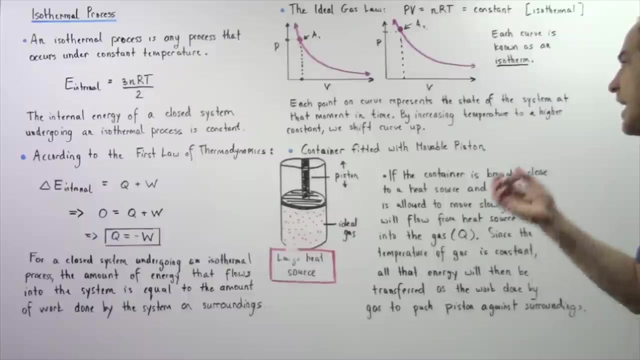 and we shift our curve downward. Now let's actually look at an example of a closed, ideal gaseous system that is undergoing isothermal process. So let's suppose we have a container fitted with a movable piston And between this space between the bottom of the container, that 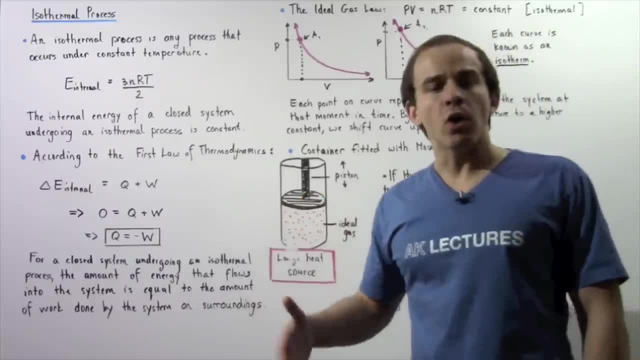 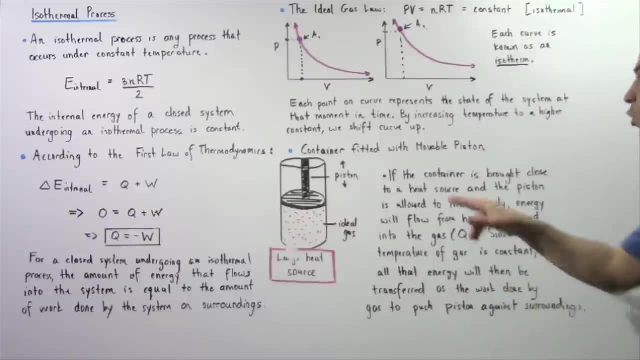 is closed and this piston, we have our ideal monatomic gaseous system. So let's suppose we have a cold gas and a cold gaseous system Now this slide suggests that the temperature of this piston will drop down to about 3 degrees. Let's say where we have a completed isotherm which is 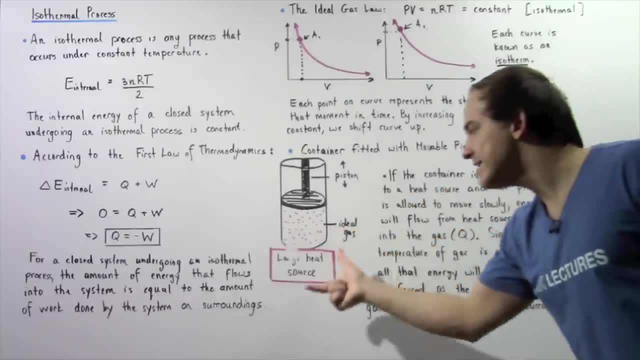 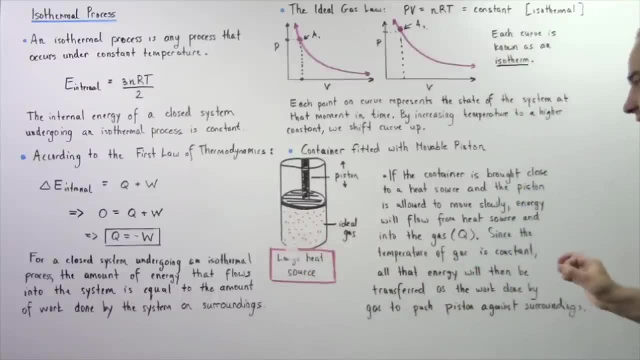 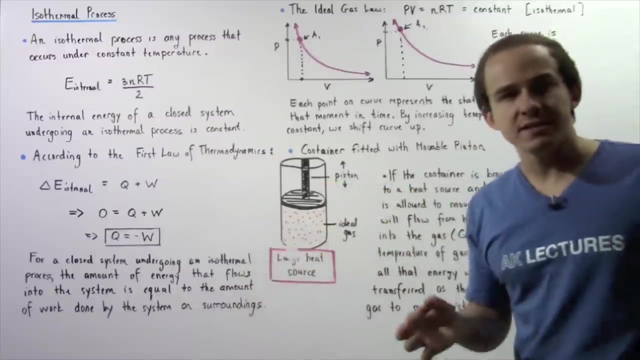 the temperature of the piston. Now we have all of these molecules in this gaseous system in the water. We can see that the temperature of the piston is 2 degrees and that the temperature is 3 degrees. So the temperature of the piston is 3 degrees, which is almost 2 degrees. Now let's 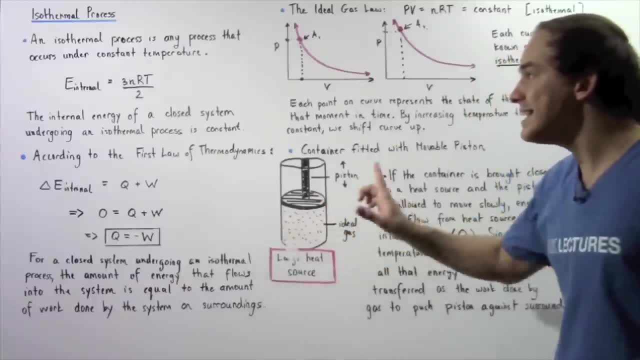 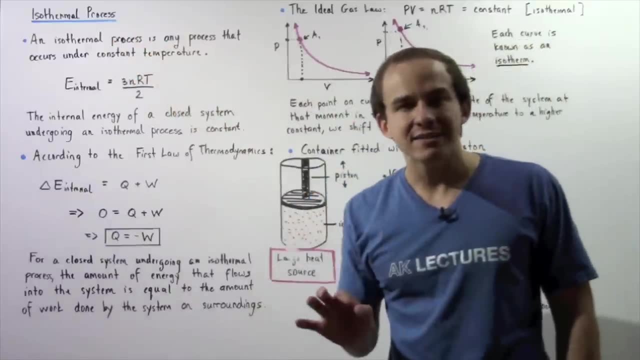 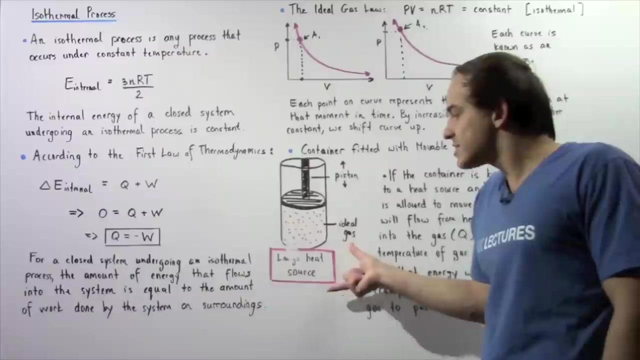 have a look at an example of a closed ideal gaseous system that is undergoing isothermal. ihnement is undergoing an isothermal process. the temperature of that ideal gas remains constant, So that means the energy that flows in to our ideal gas system from this large heat source.